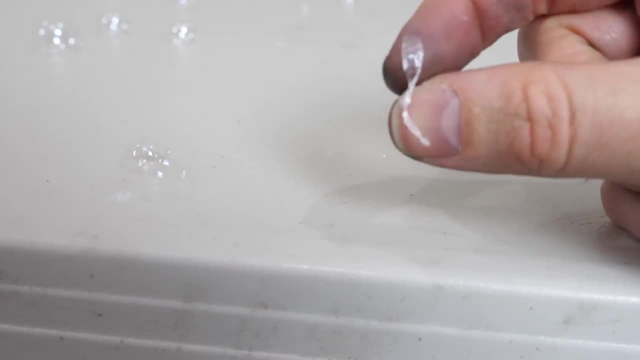 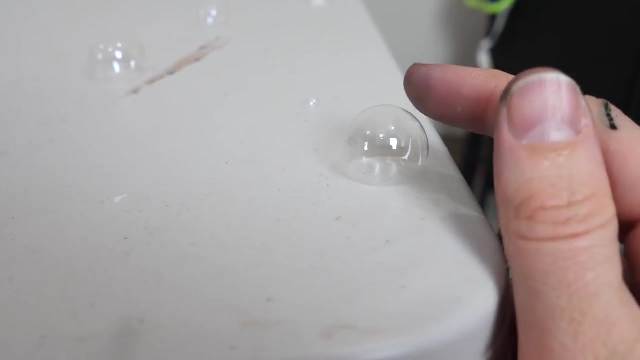 when you do pop them they're kind of sticky. They have an actual skin to them. So the reason these are able to last so long is because they don't depend on water, but a slight polymer form. They don't have a lot of film around them. 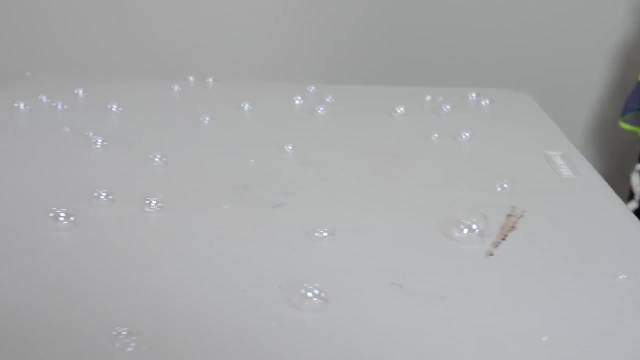 So that means you can even touch them. But the cool part is is they look just like normal soap bubbles. So the bubbles that I blew in my garage here that just landed on the table and the floor. they've been here for over five hours and still no change. 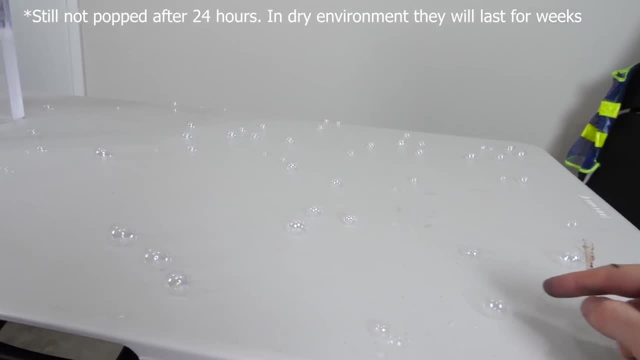 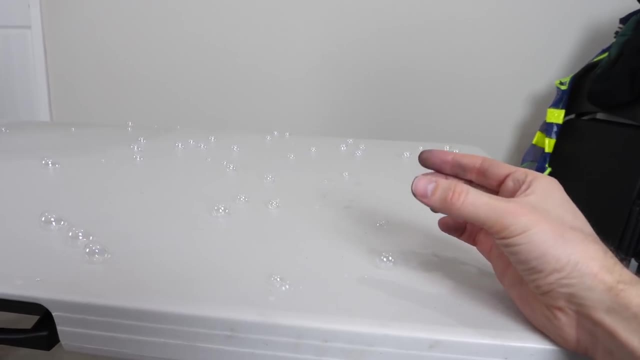 So I assume they'll just stay this way pretty much indefinitely until something pops them Normal bubbles, even if they can land like this and not pop as they dry out. they get smaller and smaller and smaller, But these keep their shape because of this polymer on the outside. 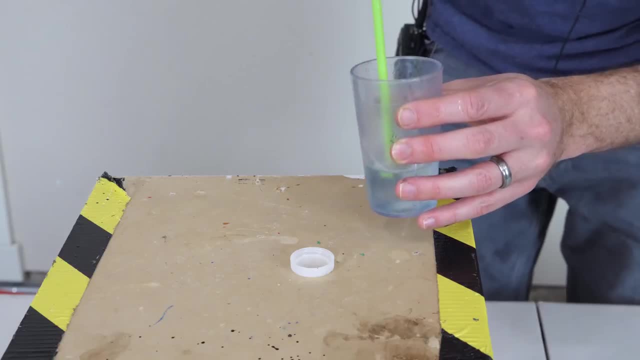 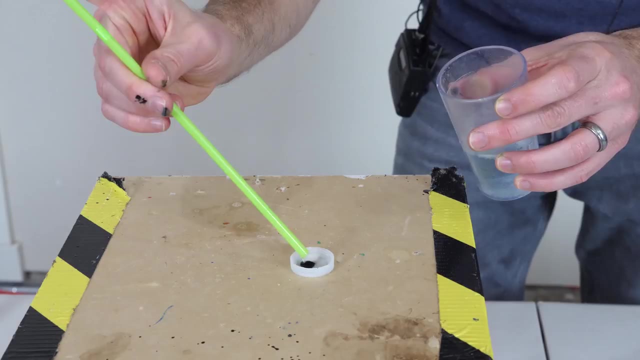 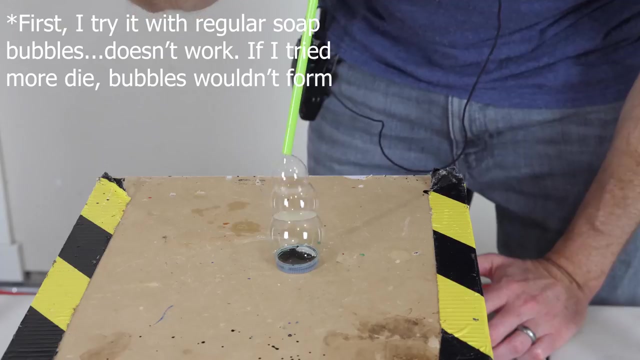 So first let's see what this looks like when I try to do it with just regular soap bubbles. So if I mix some of this black in, let's see if it works. So the bubbles work, but it doesn't look that black at all. 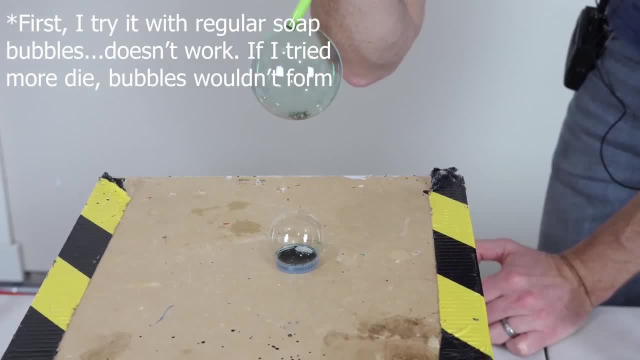 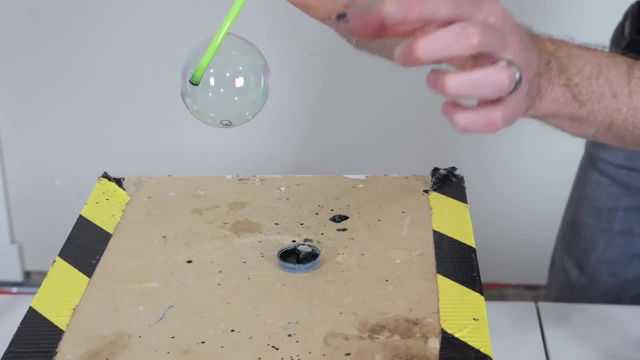 You can see that with regular soap bubbles, even though there's black paint in it, the membrane is so thin that you can't really see the black color at all. But the key to getting this to work is to get a bubble membrane that is much thicker than the normal water soap membrane. 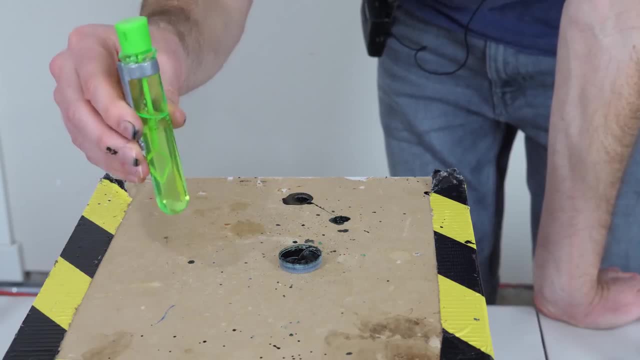 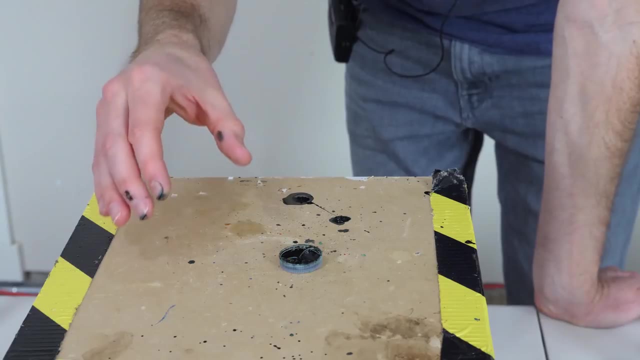 So hopefully this will be thick enough to actually be able to see the black color of the bubble. Okay, so first let's get some of our black paint and then we're going to get some of our black paint. So we're going to get some of our black paint. 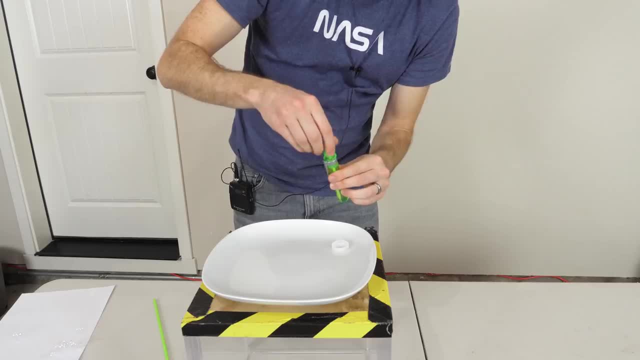 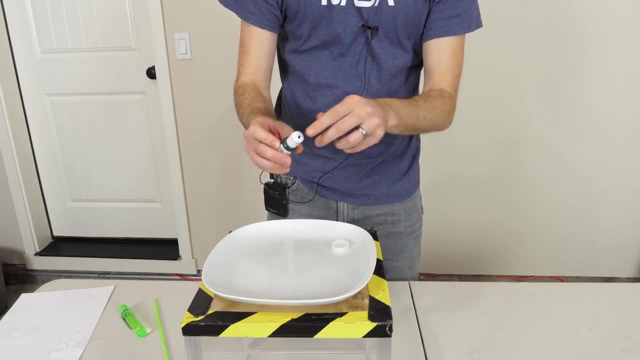 And then we're going to get some of our black paint And then we're going to get some of our bubble solution here, And then I'm going to be putting some Chef Master coal black food color in it, And this is a lot more of an intense color. 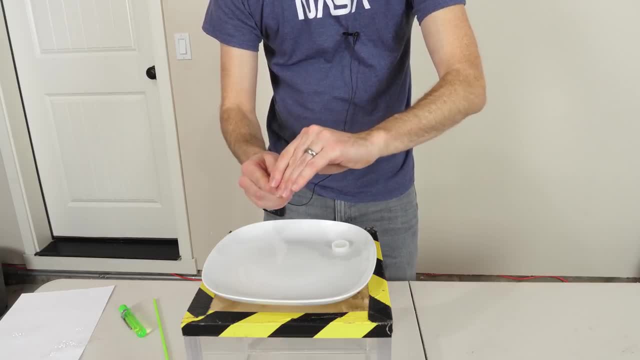 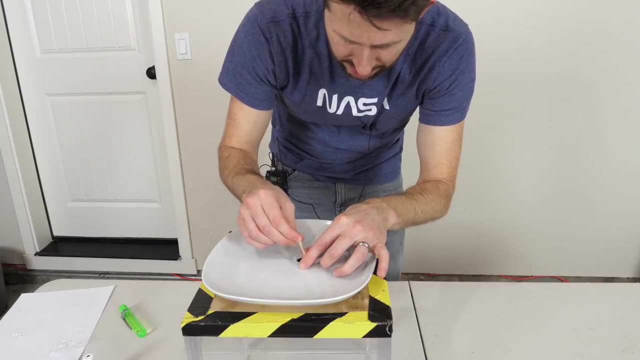 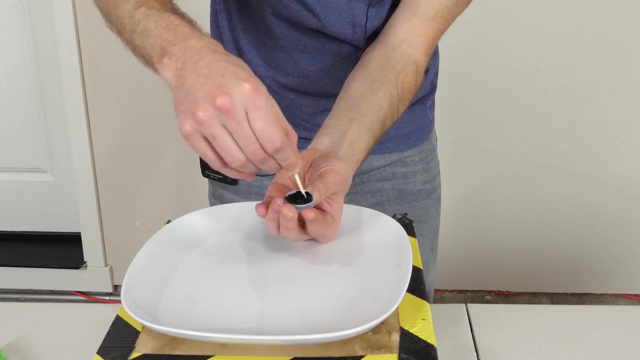 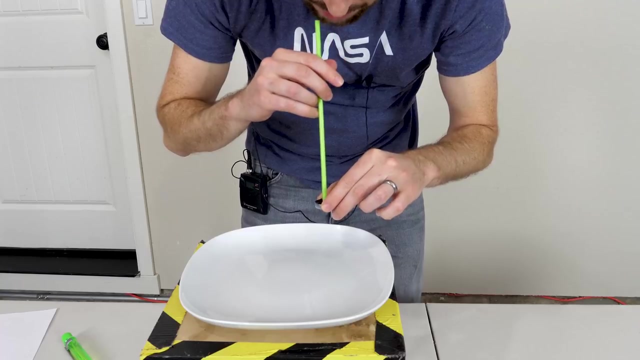 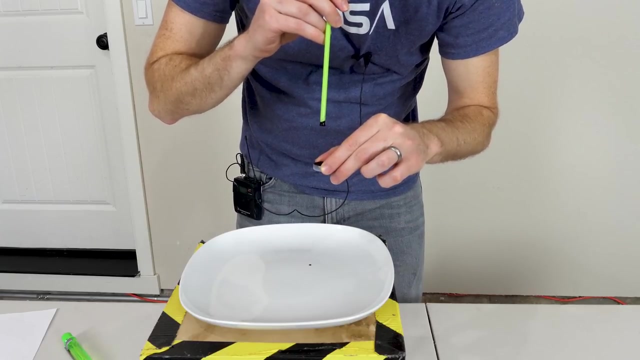 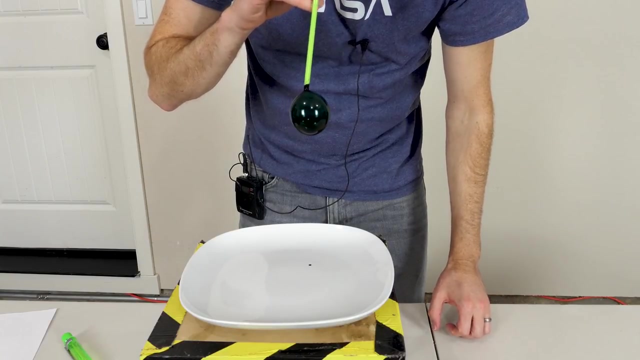 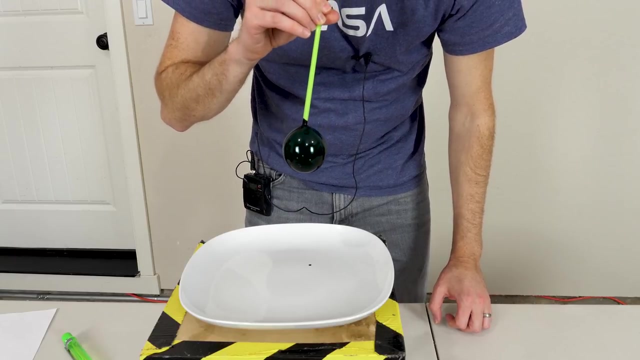 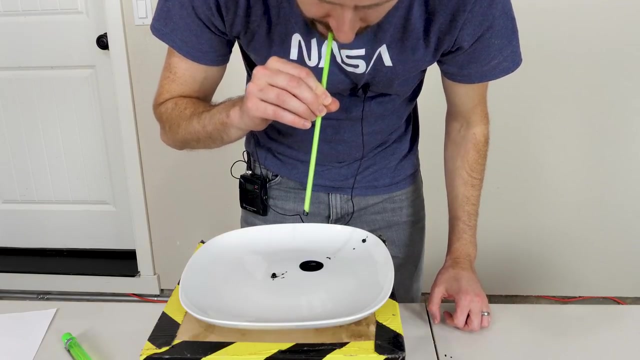 than regular food coloring. It's extremely dark. Let's add some to it. Stir it up here So you can see how black this is. now Okay, let's see if this actually works. Oh bro, it was totally black. 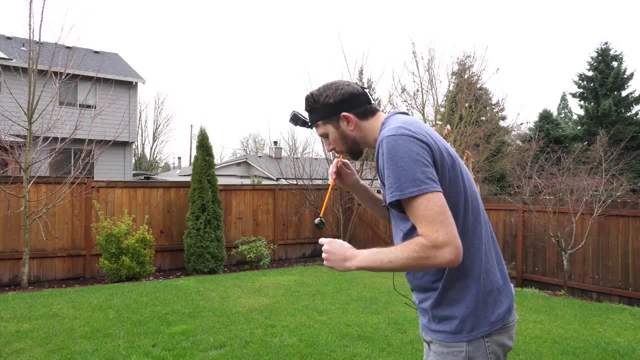 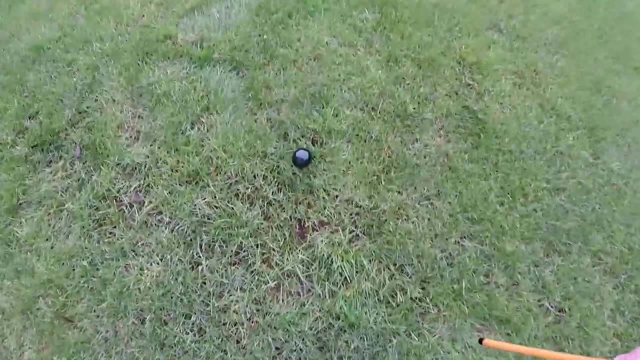 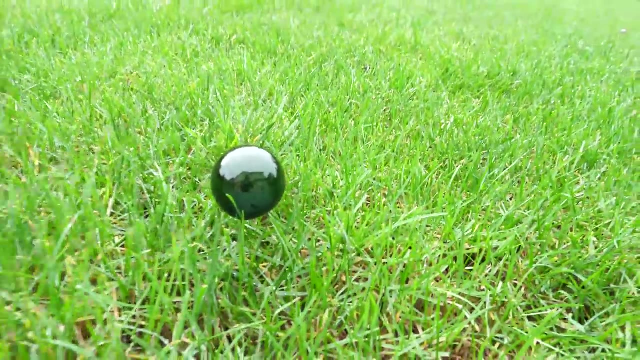 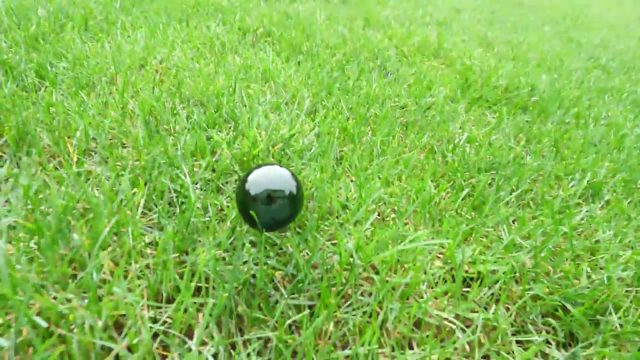 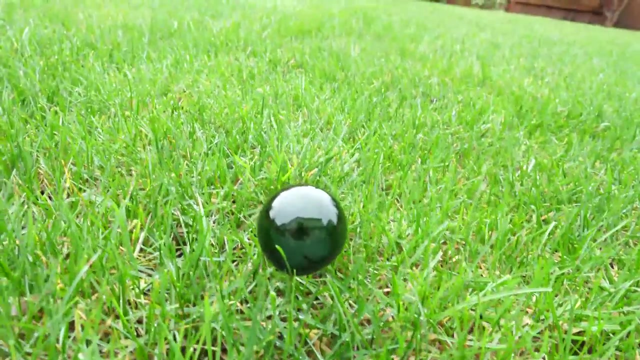 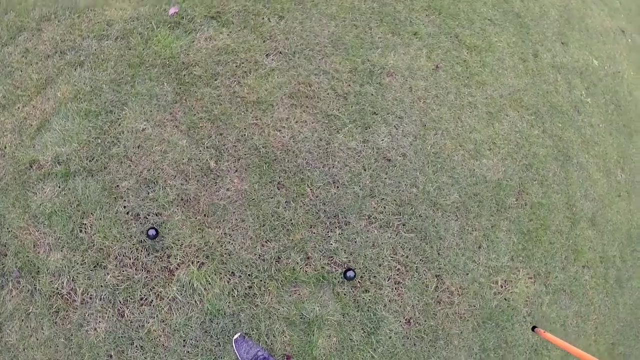 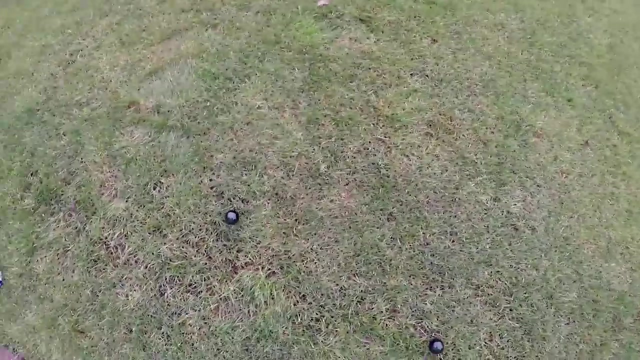 Okay, black bubble- Whoa, look at that, A black bubble. Look at a black bubble. That's so cool. It's totally black, Holy cow. look at that, So cool. Look at that one. Ha ha, Ha ha. 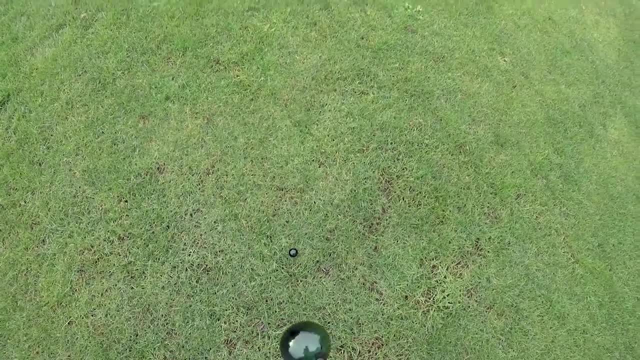 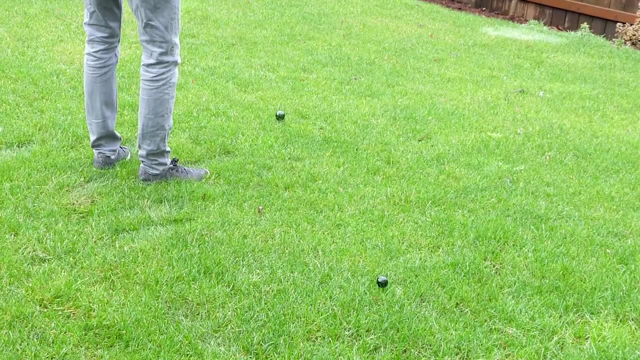 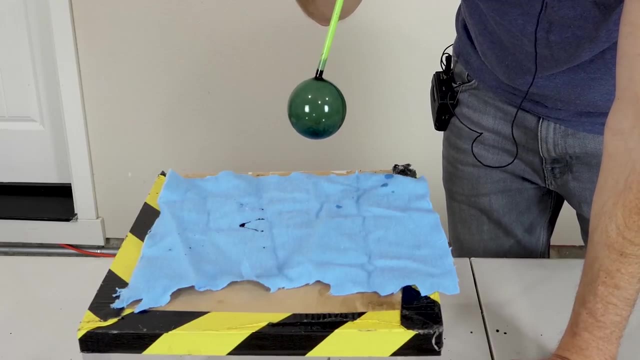 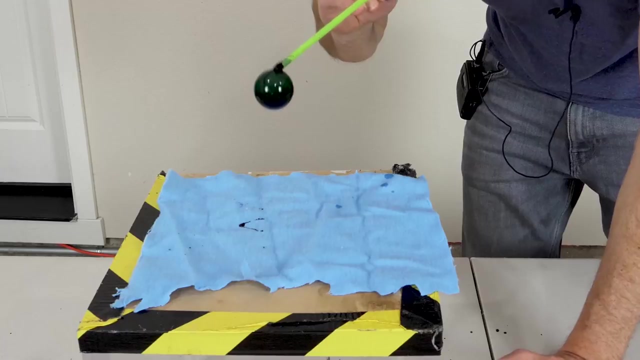 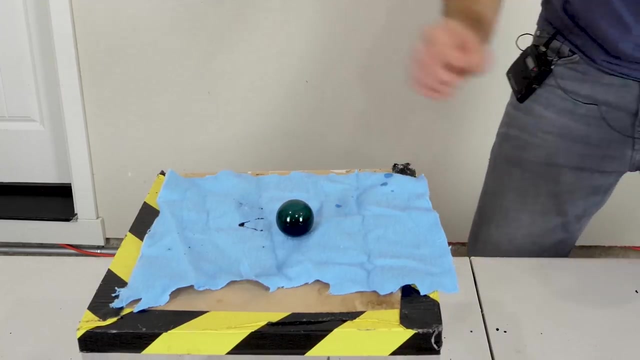 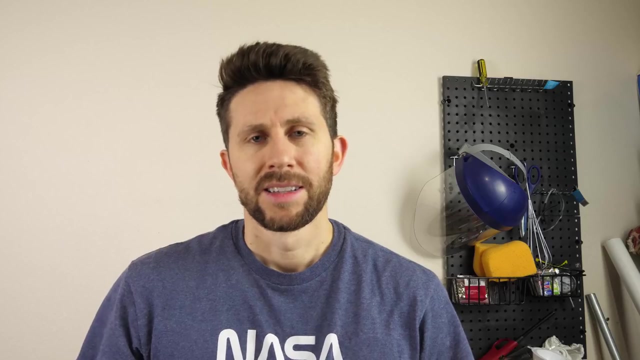 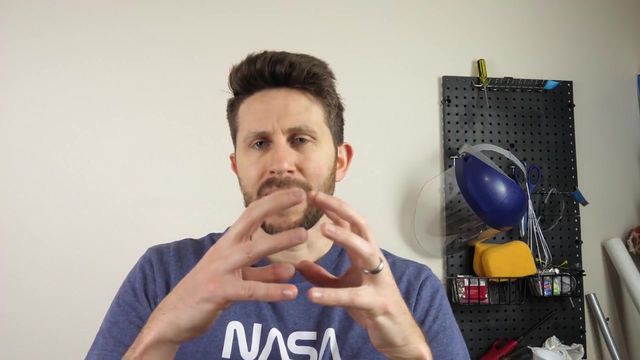 So cool. There it goes. surprised that they're actually lasting, even when landing on the grass. There we go, did it There? a self-sustained black bubble. This is actually pretty interesting. Notice that the bubble solution is extremely black, But when I blow up the bubbles it becomes more transparent. 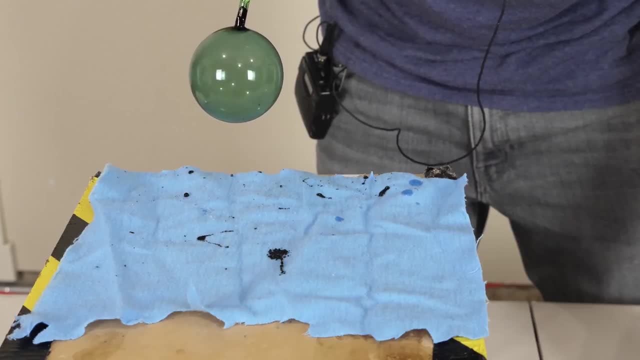 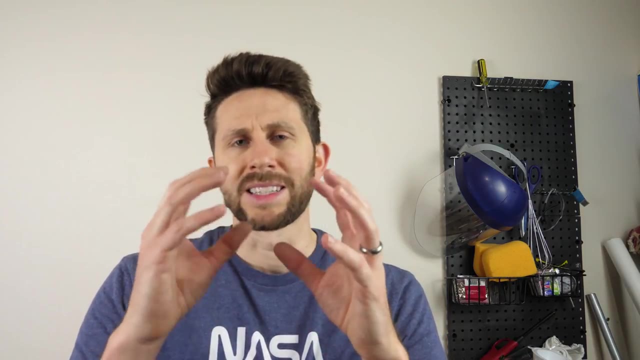 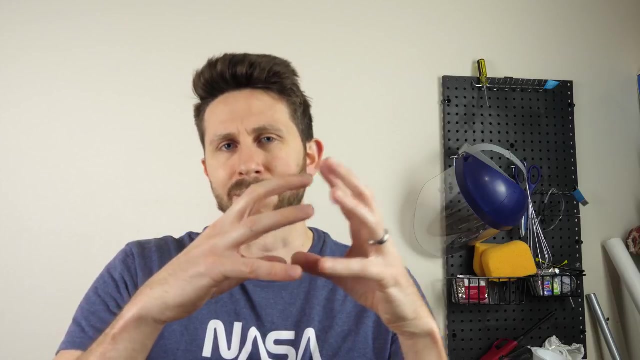 So, as the membrane got thinner, it became more and more transparent, and that's actually true for any material, even metal. Now, in the case of the bubbles, the reason that happened is because the pigment that was in the bubble solution was spreading out, So there weren't as many pigments per area, and so it looked like it was more transparent. more light was getting through. 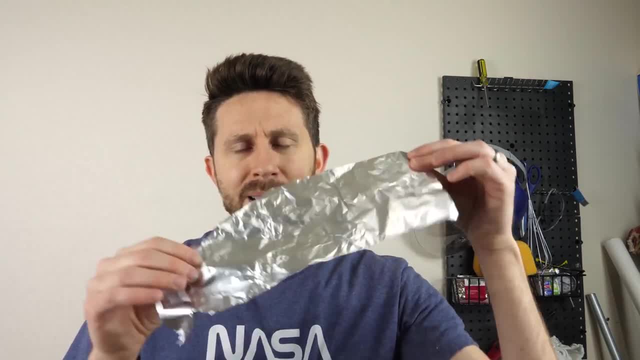 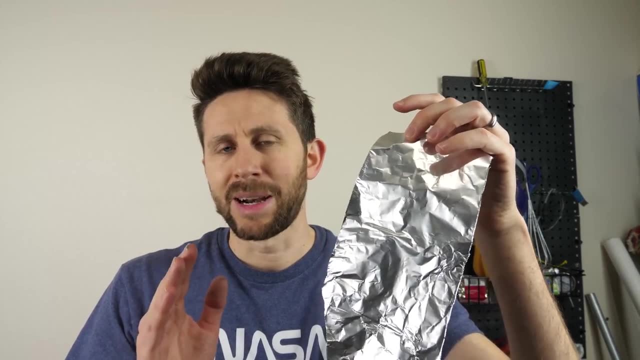 But even if you have a material that's completely homogenous, like metal Here, for example, this aluminum foil, if I was able to spread this out thin enough, would it actually become transparent too. So, for example, if I was able to pound this down thinner and thinner and thinner, 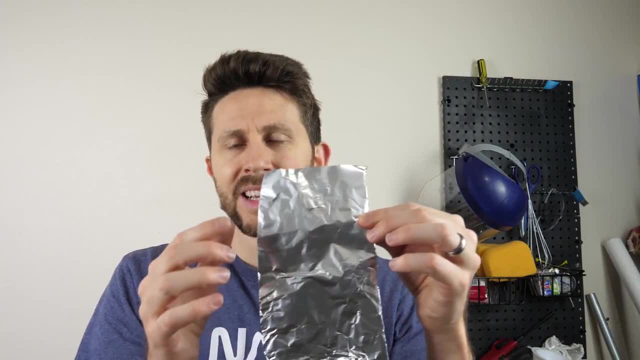 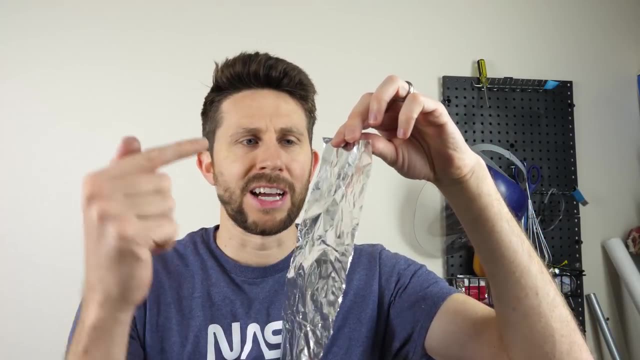 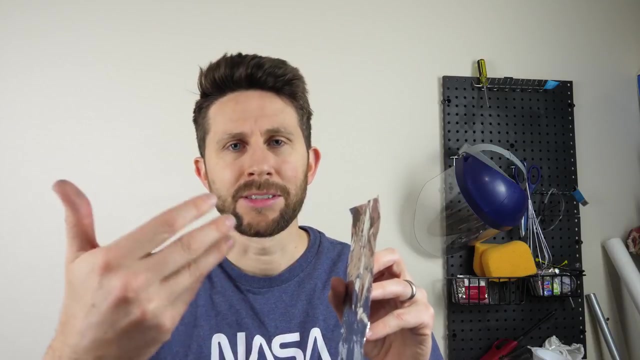 Eventually, even though I had a completely intact metal sheet, It would be transparent, completely transparent. So when light hits a metal, there's an exponential decay of the intensity of light down into the surface of the metal. So if you only have a few layers of atoms and you shine light through it, there aren't enough atoms to absorb. 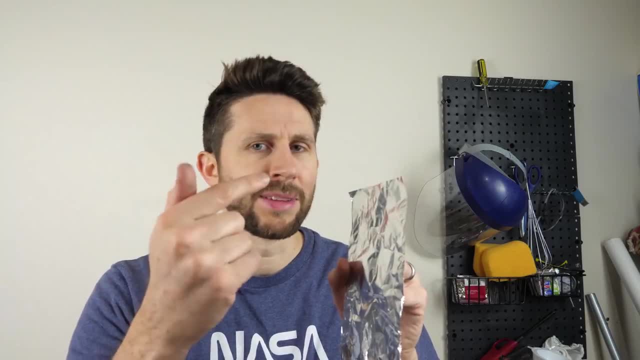 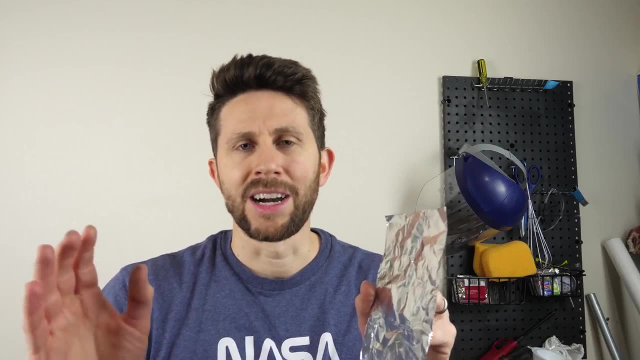 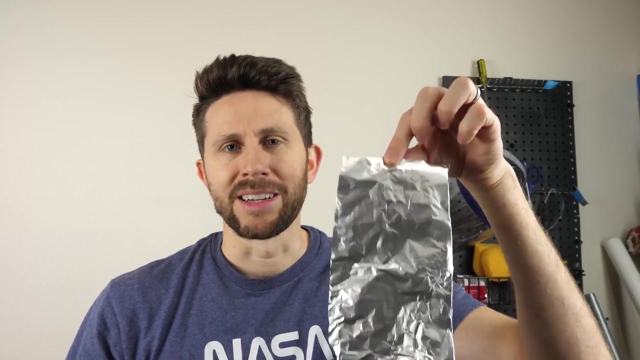 That light. so it attenuates a little bit. it absorbs some of the light, But most of it will just pass through it. But you have to be in a very thin range around 20 nanometers to a hundred nanometers thick. So around 20 nanometers of mostly any metal. it would just be completely transparent. 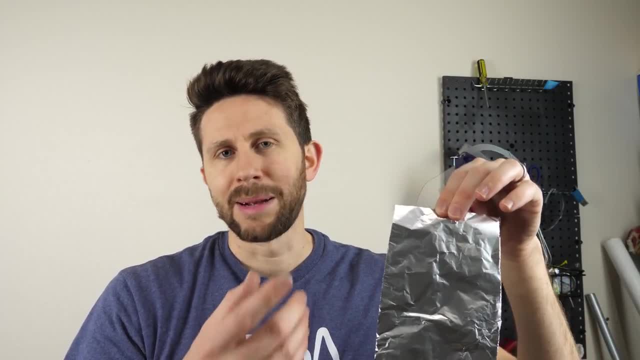 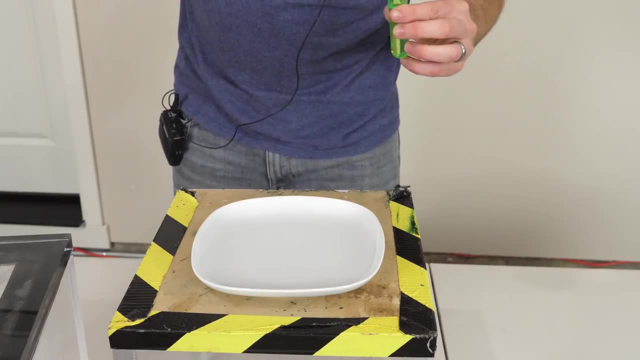 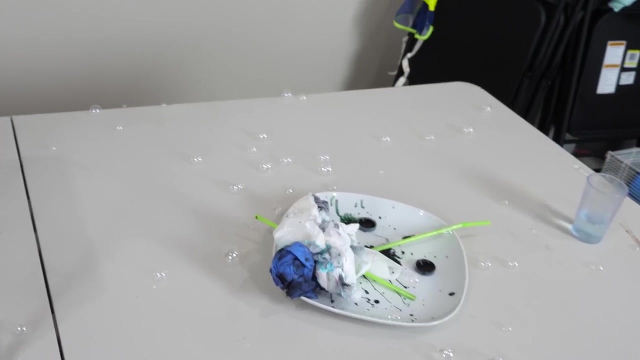 So if I had a thin enough bubble of aluminum or gold, I'd be able to see through that bubble as well. Okay, first let's get our long-lasting bubbles here. Okay, I think I finally caught enough. So I kind of have bubbles all over me after catching these. 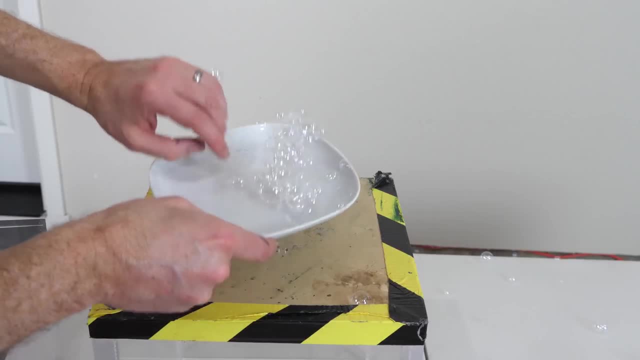 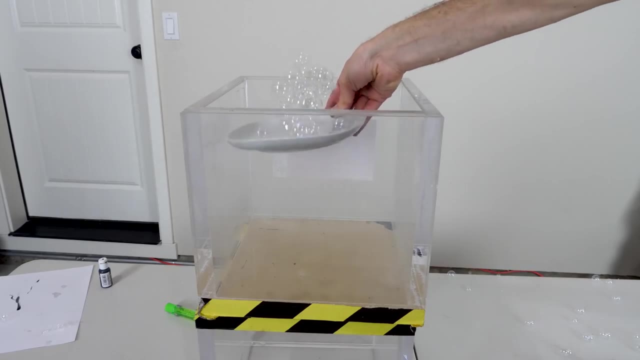 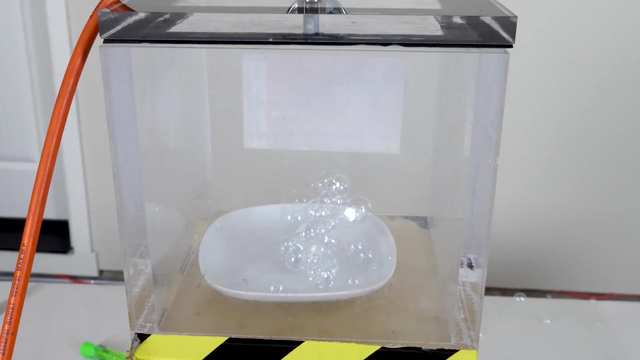 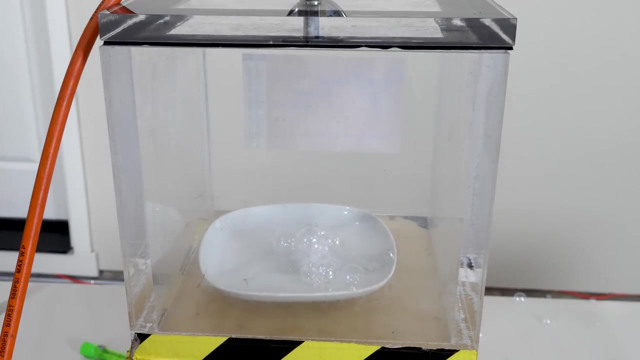 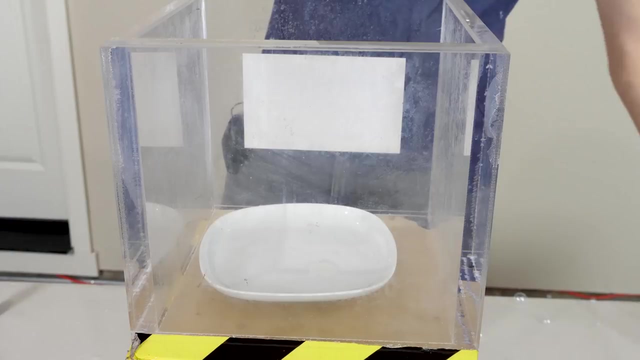 Let's see what happens in the vacuum chamber. Okay, here we go. Okay, three, two, one. Oh, They're expanding in form. Okay, I think I finally caught enough. Okay, three, two, one, They're popping. So because the bubbles dried already as soon as they started to expand, they just popped.